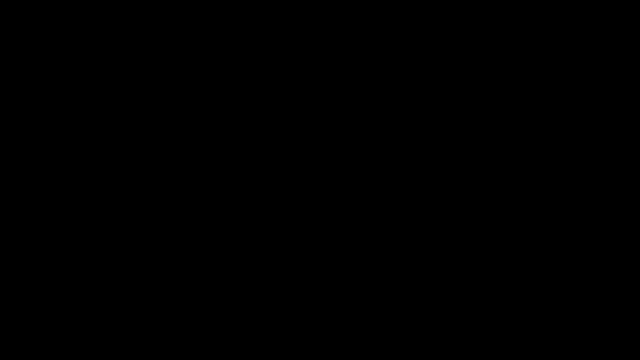 In this video we're gonna do a few examples finding domains of functions. So let's say that we have the function f of x is equal to x plus five over x minus two. What is going to be the domain of this function? Pause this video and try to figure that out. 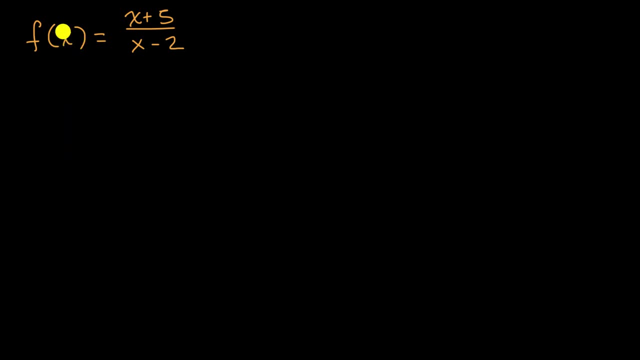 All right, now let's do it together. Now the domain is the set of all x values that, if we input it into this function, we're going to get a legitimate output, We're going to get a legitimate f of x, And so what's a situation where we would not? 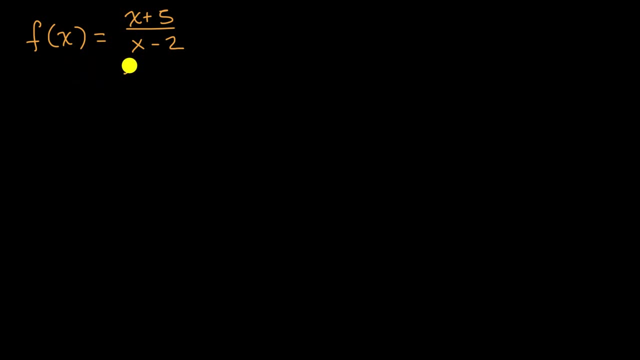 get a legitimate f of x. Well, if we input an x value that makes this denominator equal to zero, then we're going to divide by zero and that's going to be undefined. And so we could say the domain- the domain here is all real values of x. 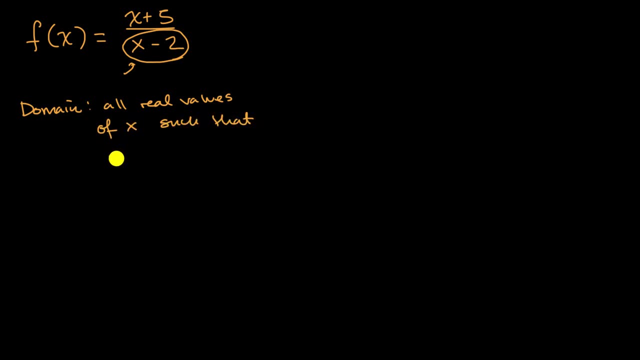 such that x minus two does not equal zero. Now, typically, people would not wanna just see that such that x minus two does not equal zero, And so we can simplify this a little bit so that we just have an x on the left-hand side. 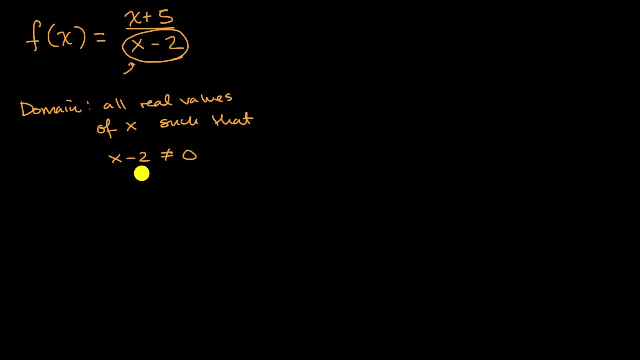 So if we add two to both sides of this, we would get actually. let me just do that, Let me add two to both sides. So x minus two, not equaling zero, is the same thing as x not equaling two, And you could have done that in your head as well. 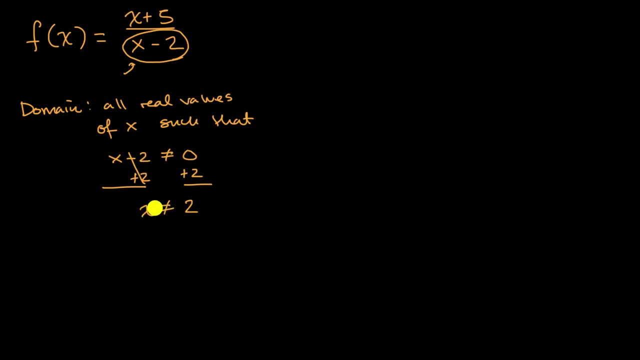 If you wanted to keep x equaling zero, right x minus two from being zero, x just can't be equal to two, And so typically people would say that the domain here is all real values of x, such that x does not equal two. 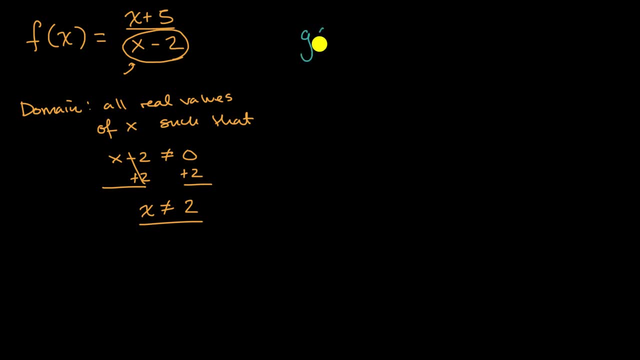 Let's do another example. Let's say that we're told that g of x is equal to the principal root of x minus seven. What's the domain in this situation? What's the domain of g of x? Pause the video and try to figure that out. 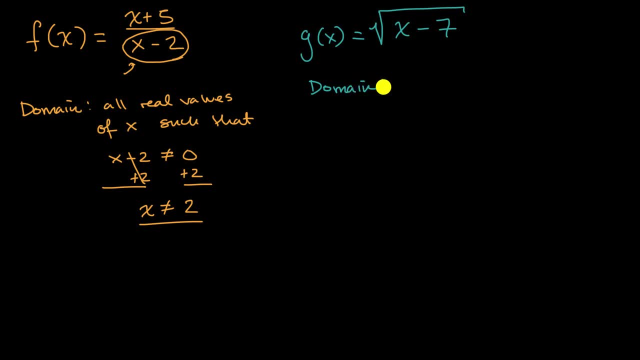 Well, we could say that domain, the domain is going to be all real values of x, such that are we gonna have to put any constraints on this? Well, when does a principal root function break down? Well, if we tried to find the principal root, 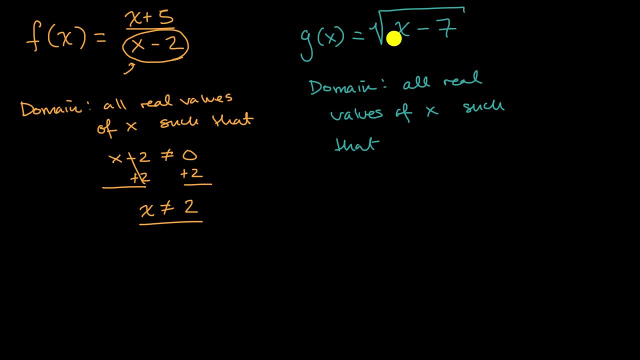 the square root of a negative number. well, that would then break down, And so x minus seven- whatever we have under the radical here- needs to be greater than or equal to zero, So such that x minus seven needs to be greater than. 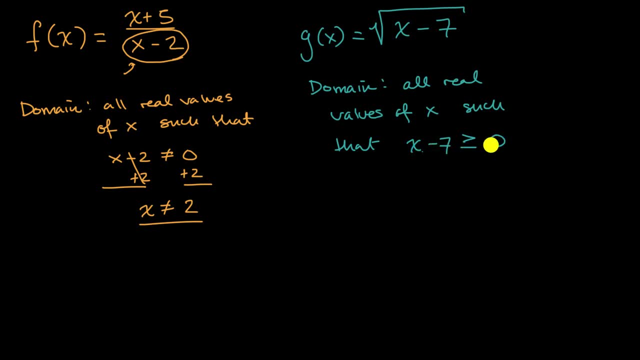 or equal to zero. Now another way to say that is: we add seven to both sides of that. That would be saying that x needs to be greater than or equal to seven. So let me just write it that way. So such that x is greater than or equal to seven. 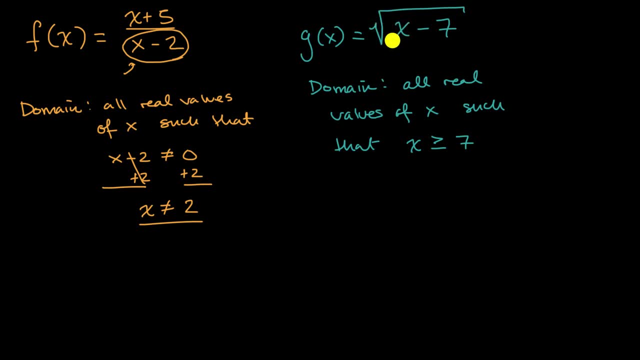 So all I did is I said: all right, where could this thing break down? Well, if I get x values, I could break down this right. where this thing is negative, we're in trouble. So x needs to be greater, x minus seven. 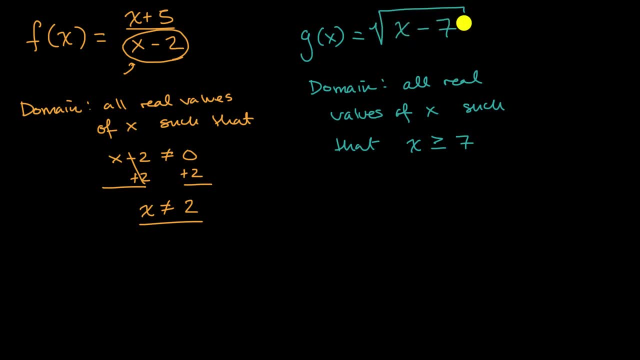 whatever we have in this under the radical- needs to be greater than or equal to zero. And so if you say that x minus seven needs to be greater than or equal to zero, you add seven to both sides. you get x needs to be greater than or equal to positive seven. 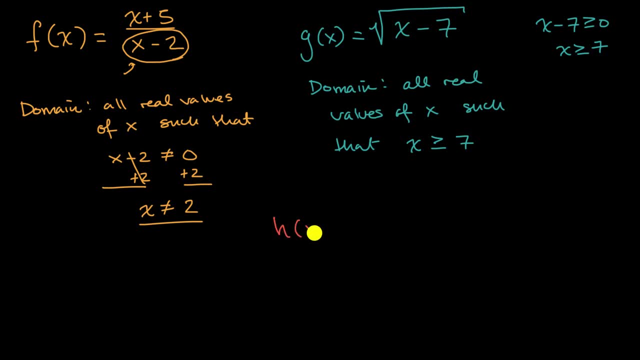 Let's do one last example. Let's say we're told that h of x is equal to x minus five squared. What's the domain here? So let me write this down: The domain is all real values of x. Now are we going to have to constrain this a little bit? 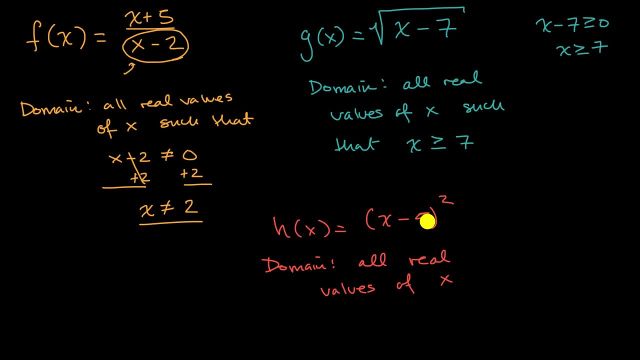 Well, is there anything that would cause this to not evaluate to a defined value? Well, we can square any value. You have to give me any real number, and if I square it, I'm just gonna get another real number. And so x minus five. 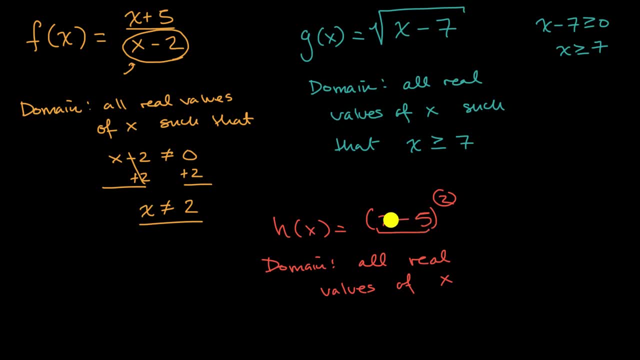 can be equal to anything, And so x can be equal to anything. So here the domain is all real values of x. We didn't have to constrain it in any way like we did the other two- The other two when you deal with something. 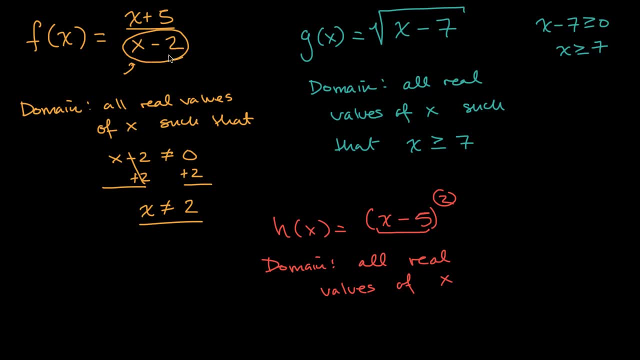 in a denominator that could be equal to zero, then you gotta make sure that that doesn't happen, because that would get you an undefined value, And similarly for a radical. you can't take the square root of a negative, And so we would once again have to constrain on that.